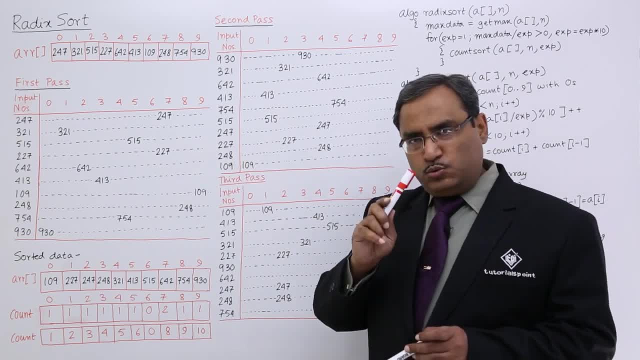 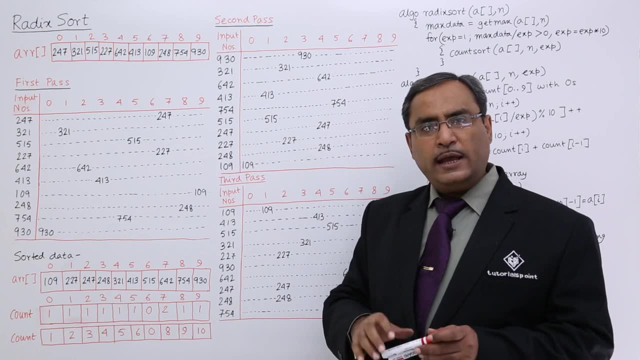 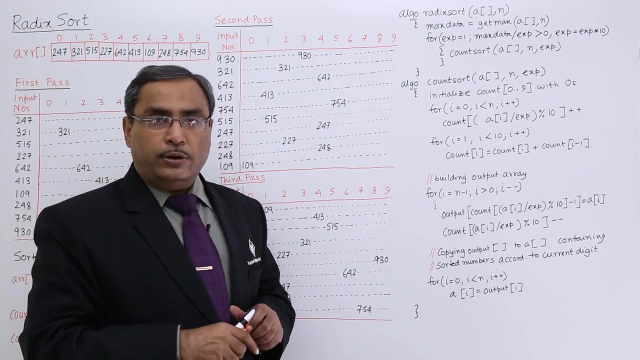 discussed this one with one example. Please watch that video, because this video is in the continuation of the previous one. Now, in this particular video, we shall go for the algorithm: How this thing can get implemented. Now see, this is my radix shot algorithm. 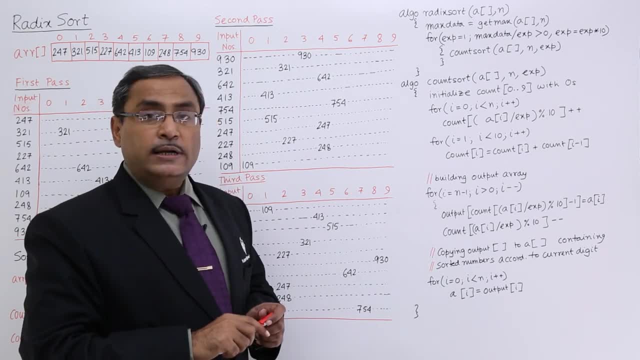 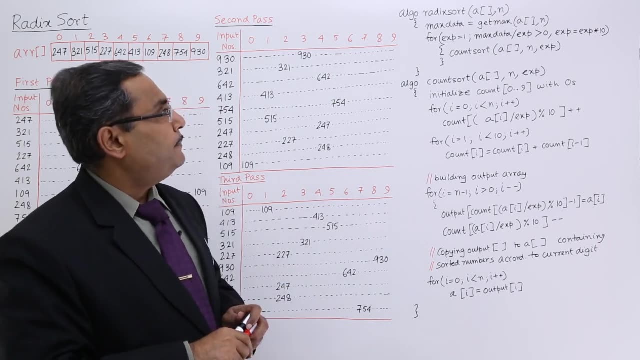 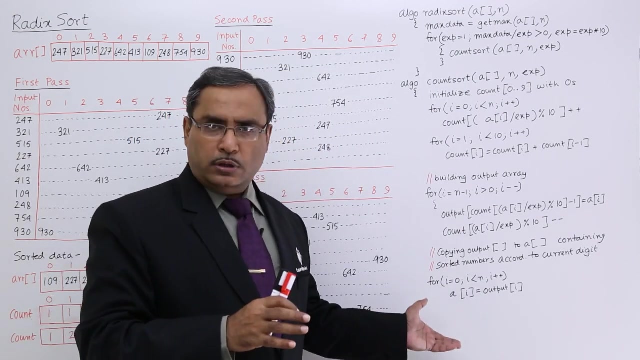 So algo radix shot a n. What is a? That is the name of the array containing our n number of data unshotted. obviously, Max data is equal to get max a n. So get max is nothing but a function. I have not shown the 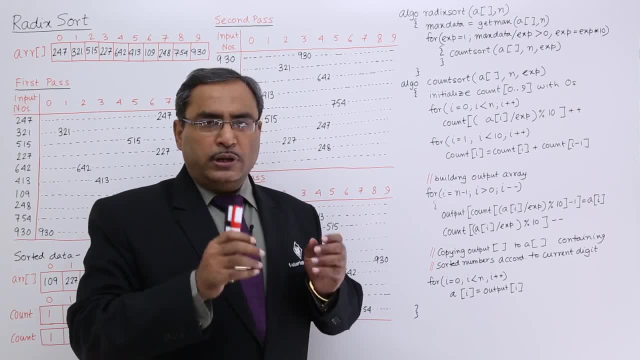 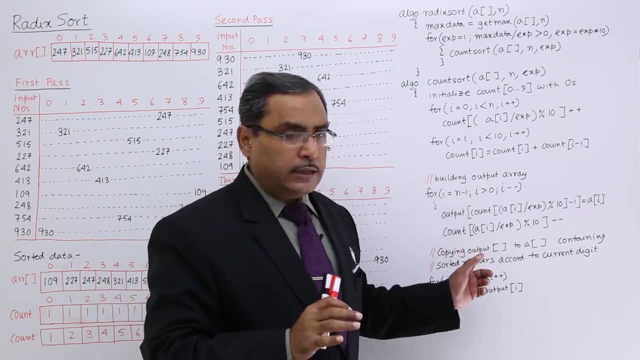 code here, because the code is very simple, which will calculate or which will find out the maximum number out of n number of numbers. So I have not written the code for get max, but I think anyone can write. So get max is nothing but a function which will take. 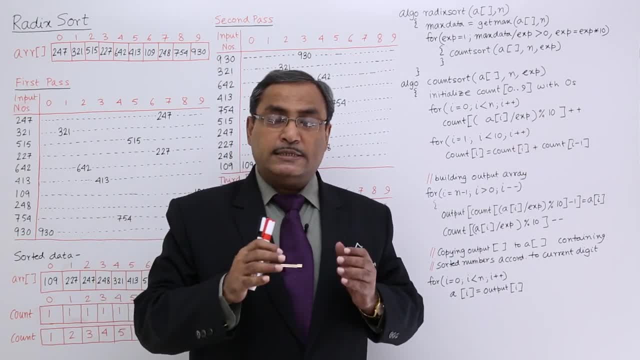 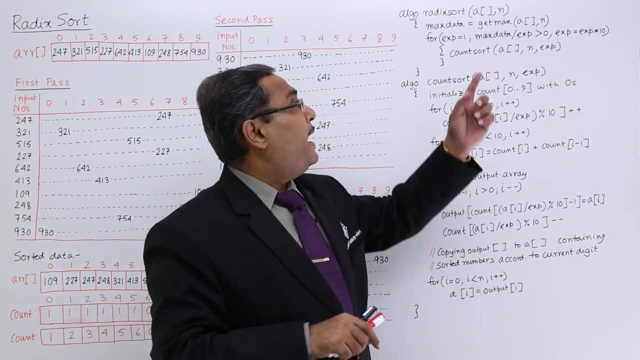 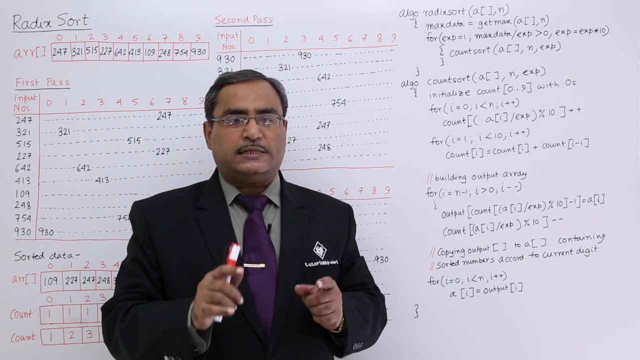 a and n as input, and then it will find out the maximum data out of n number of numbers residing in the array a. You might be asking me what is the purpose of finding this max data? because depending upon the max data, we can easily understand that how many digits are there in maximum in a single number and 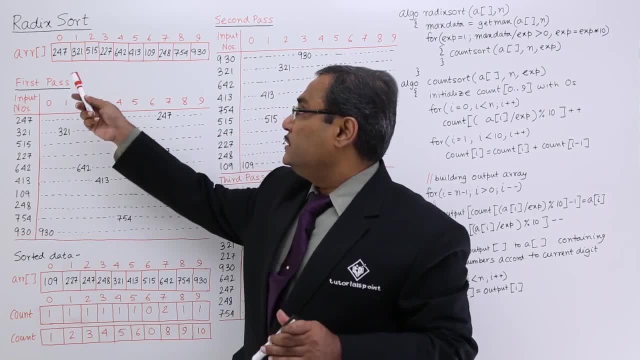 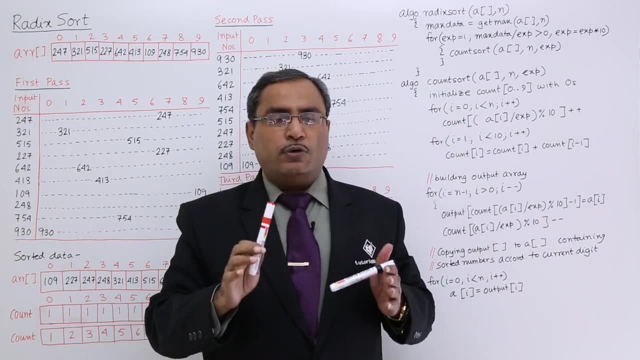 that will decide the number of passes required. Here I consider all numbers with three digit numbers. So that is why I required three passes. but if I am I was, having, say, four digit number maximum, then I shall be requiring four passes. So that is why this max data. 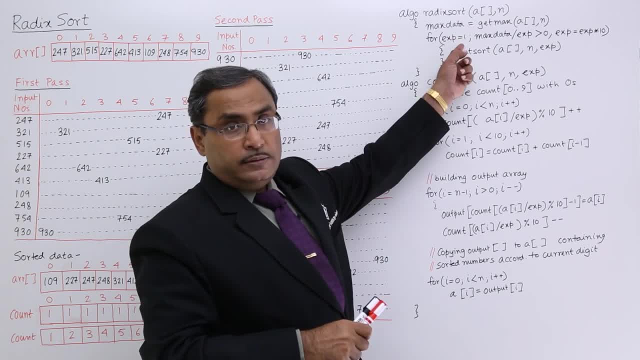 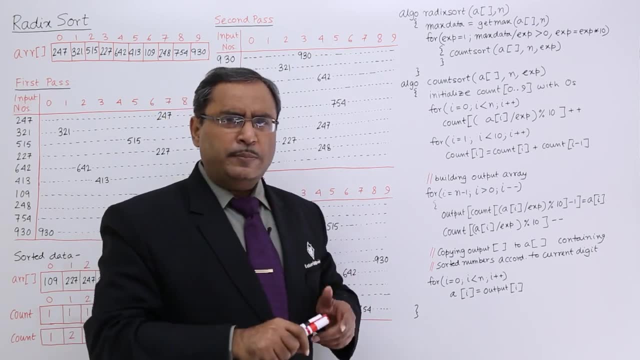 is required Now for exp. 1. exp is equal to 1 max data by exp greater than 0, exp is equal to exp into 10.. Let us suppose I am taking one data: 4,, 5,, 6. So exp is equal to 1 at. 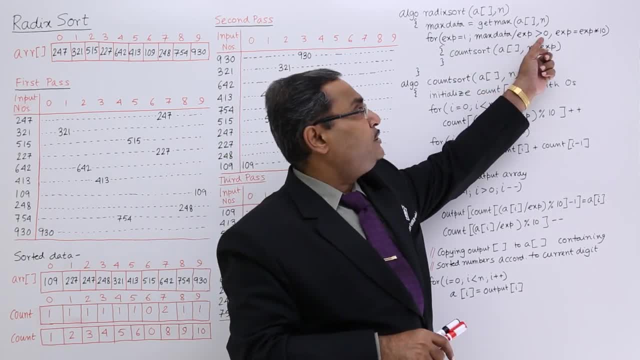 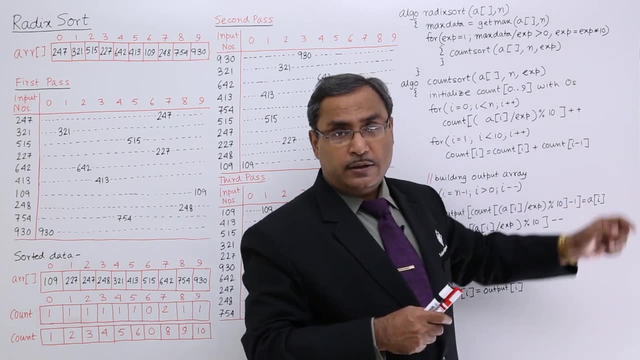 first. So 4, 5, 6 by 1 is equal to 4, 5, 6, greater than 0 is true. So count shot will be called and exp is getting increased by multiplication by 10.. So next time the value. 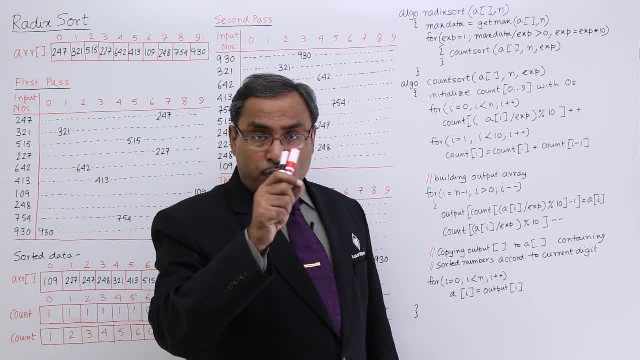 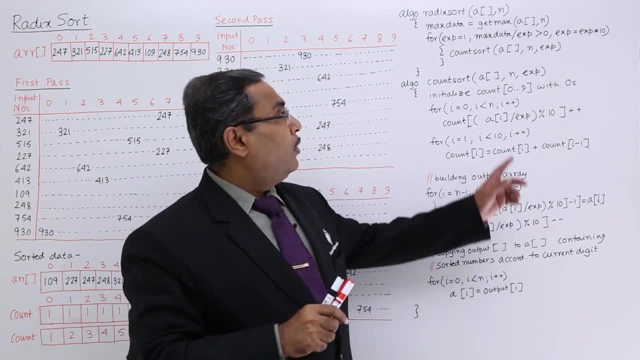 of exp will be 10,. 1 into 10 is equal to 10.. So 4, 5, 6 by 10 is 45, by 45.6 is greater than 0. So second time count shot will be called. 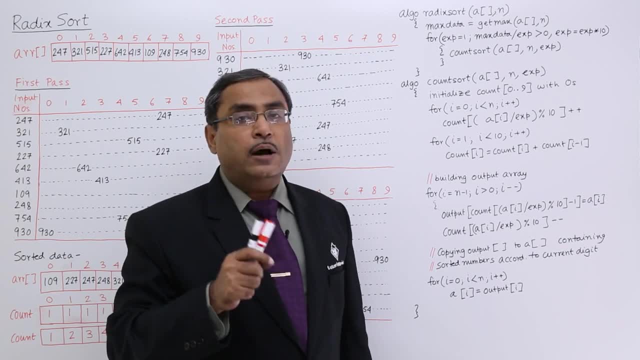 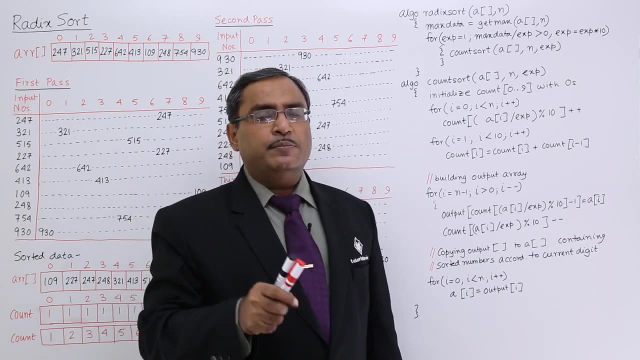 Now consider the third time. So 4, 5, 6. by now it is 100.. So 4 by 4, 5, 6 by 100, now it is becoming 4.56, as I am considering the integer one. So it is 4 and 4 is greater. 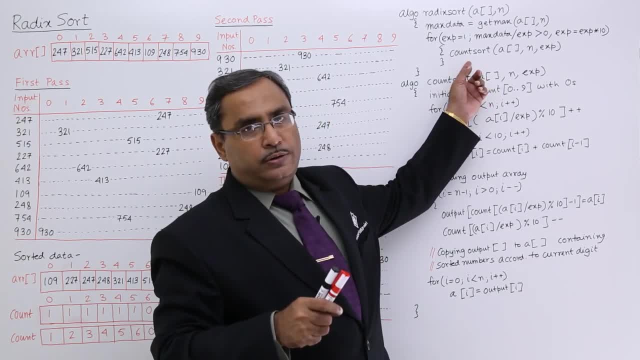 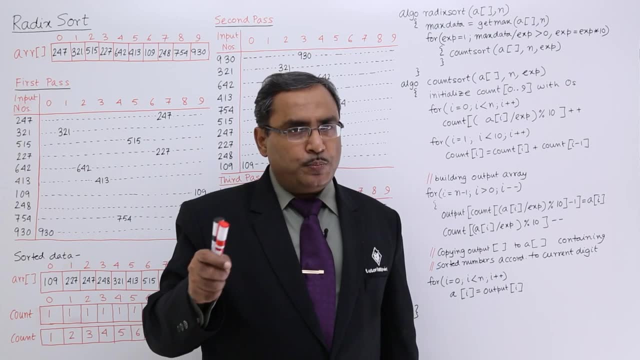 than 0 is true. So for the third time, count shot will be called. but when the value of exp will become 1000, then 4,, 5, 6 by 1000 is equal to 0.456, as this particular max data. 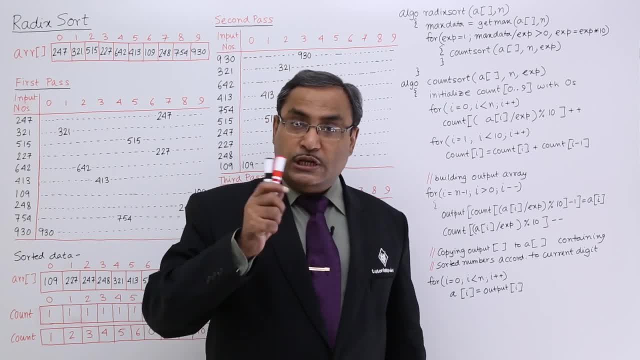 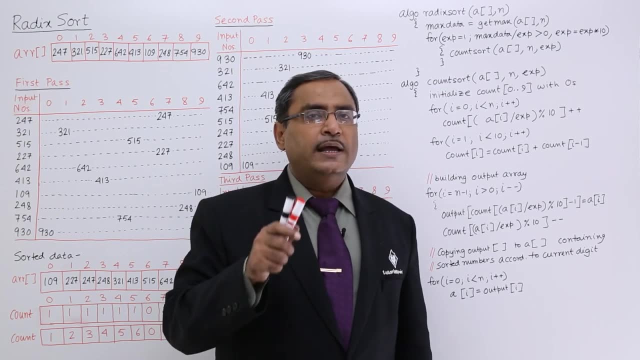 is of the type integer, I shall be remaining with 0. So 0 is greater than 0 is false. So count shot will not be called. So 3 times count shot will be called because 4,, 5, 6 was having 3 digits, So that 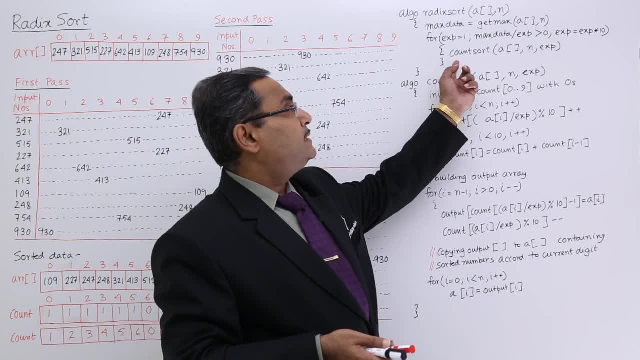 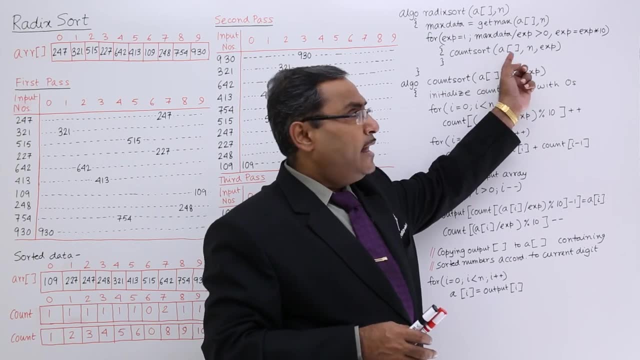 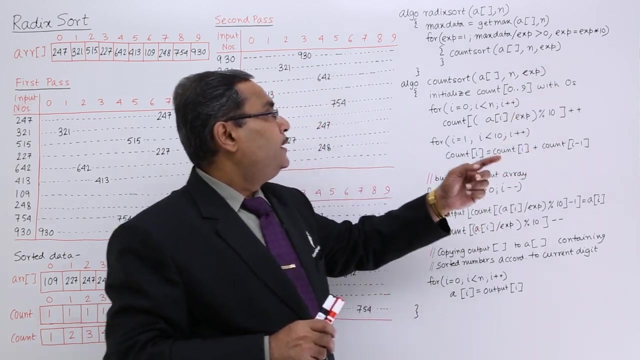 is the purpose of this. So I am remaining with one task to discuss this count shot. Count shot is taking this array as input, The number of data deciding in this array and the exp, whether it is 1 or 10 or 100 or 1000 and so on. 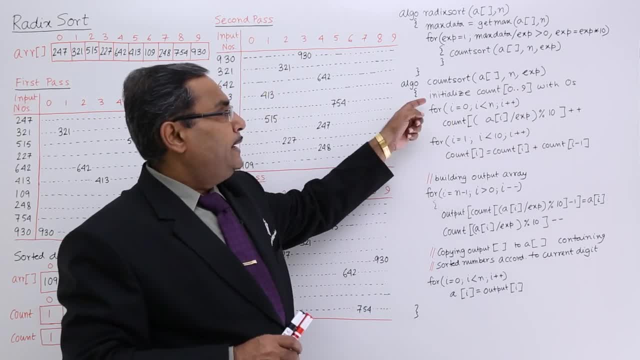 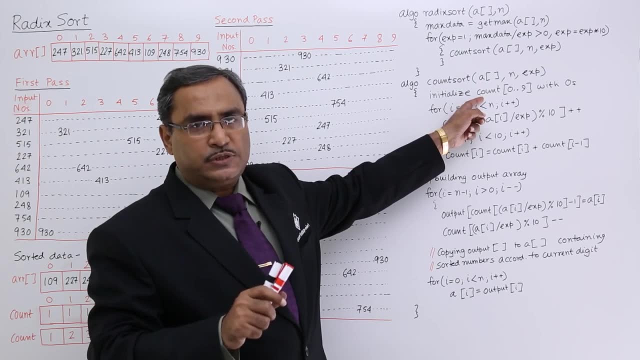 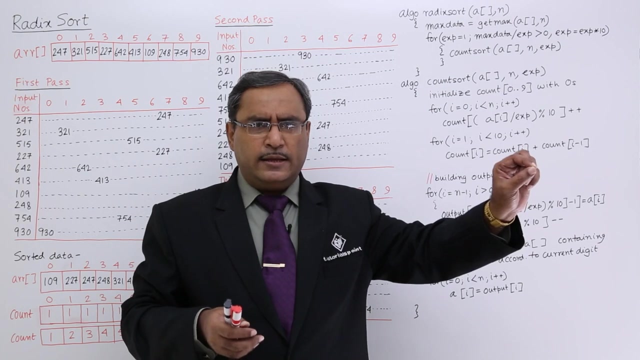 So count shot is accepting those input parameters. Now see initialize count. So that is another separate array count. having got 10 locations, 0 to 9, subscript with 0s, I can execute one for loop to make them 0s, or during declaration of the array, depending upon the language in. 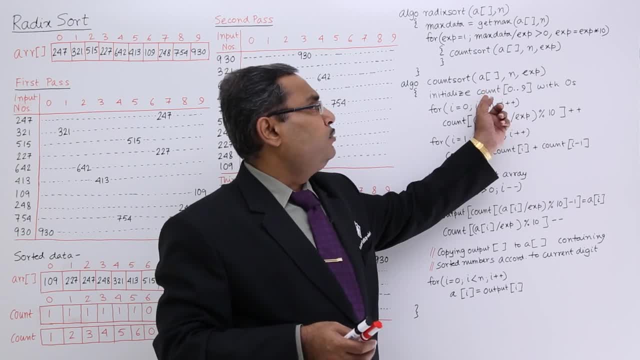 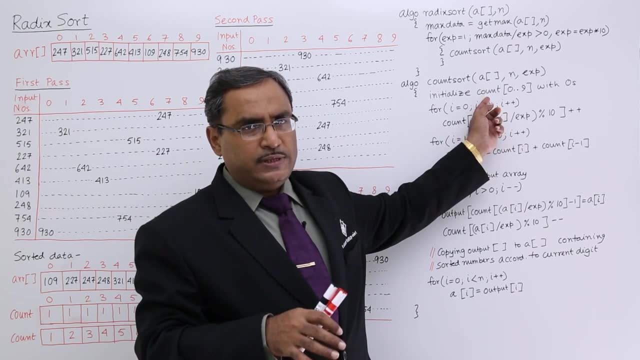 which you are going to implement. you can write the code So that this count array having 10 consecutive locations- subscript is ranging from 0 to 9- will get initialized with 0s. So count shot is accepting those input parameters Now. 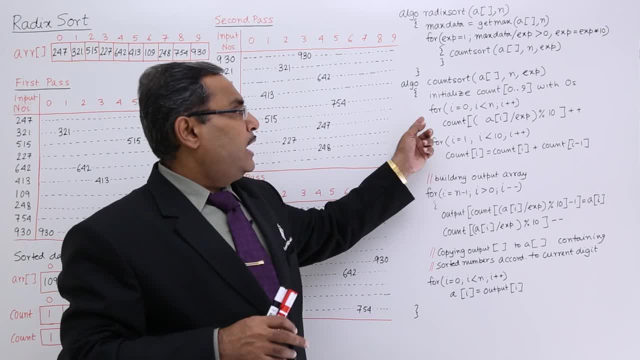 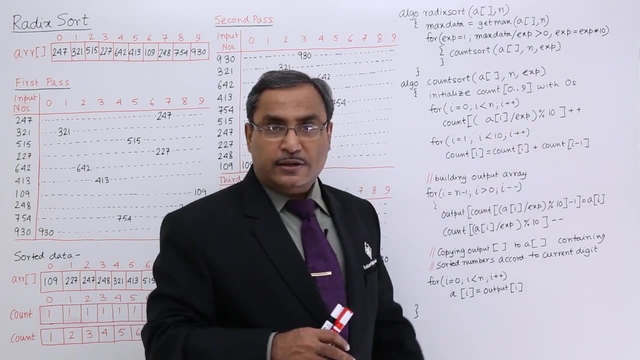 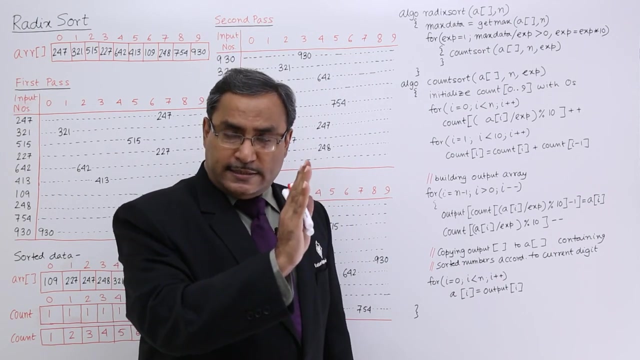 I am remaining with 0s at all locations, For i is equal to 0, i less than n, i plus plus a, i by exp percentage, 10.. So, depending upon the value of exp, whether I am going to retrieve the last digit or the second last or the third last, So that will be decided. So, depending, 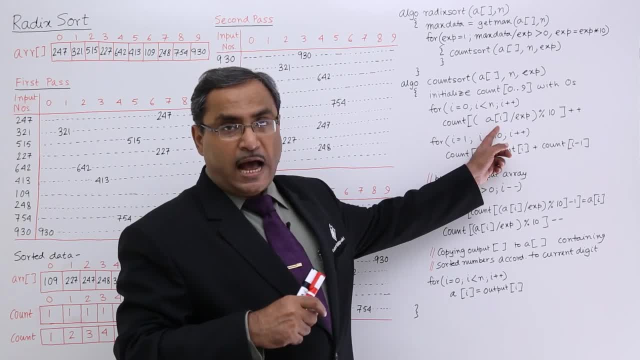 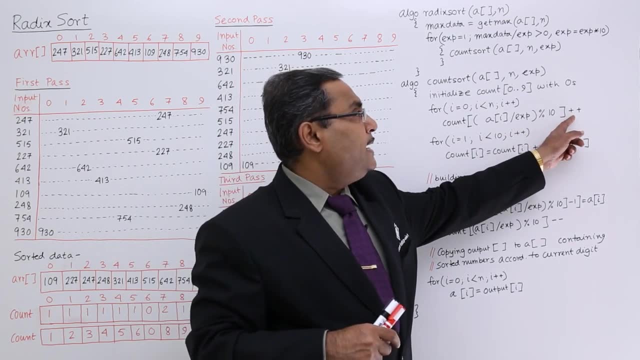 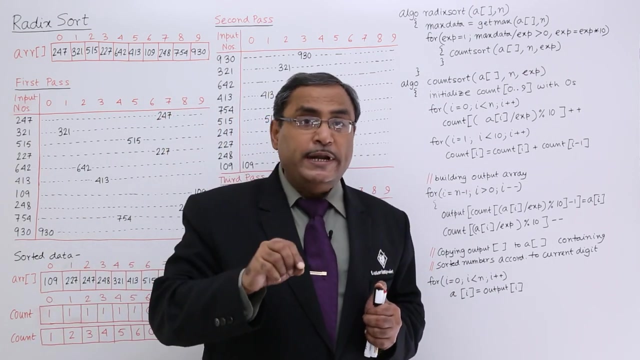 upon that digit. whatever I am retrieving from this a, i, where i is ranging from 0 to n minus 1.. So that means a respective location number will get increased. initially, count array was containing 0s, So that means with that particular digit, how many numbers are there? So, depending, 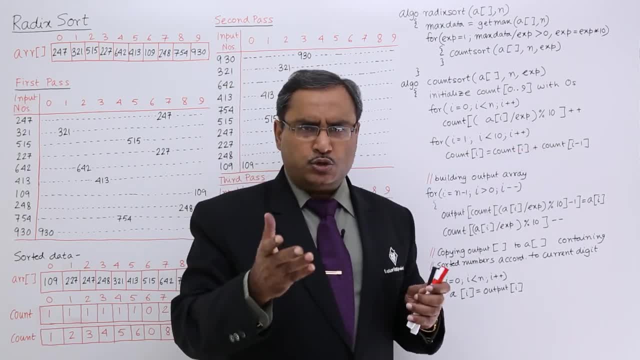 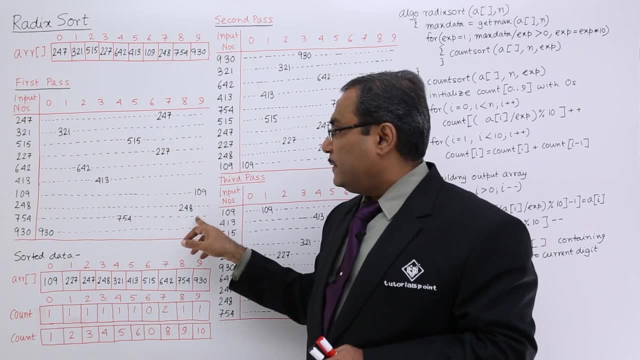 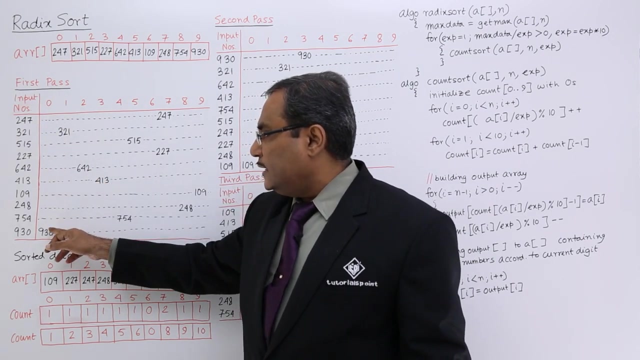 upon that, the count array will get initialized. Let me show you one example. Let us suppose this is my set of data. This is my set of data, So this is my, this particular array is this one? that means the arrangement? ok, Now see, with a 0 digit, how many digits are. 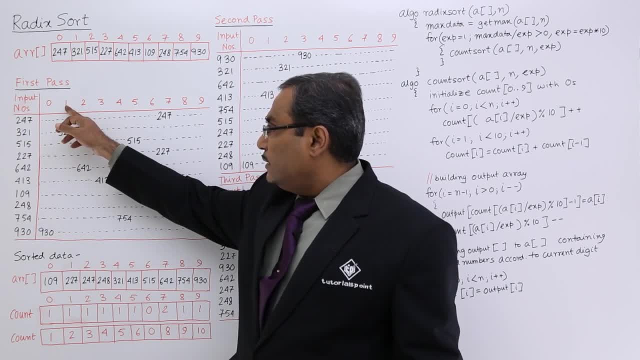 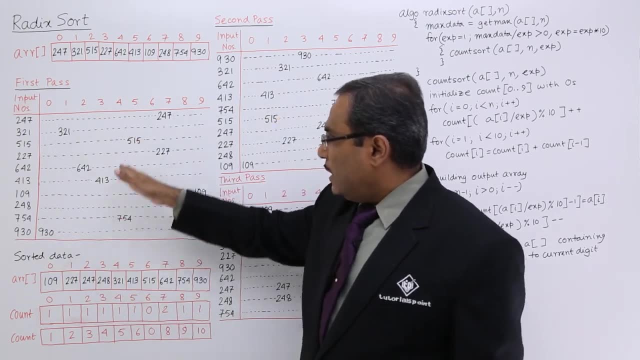 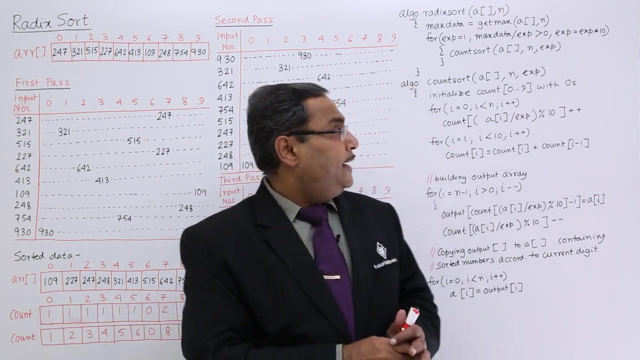 there. So I am putting there 1 with one last digit, 1-1 number. So last digit, 2-, 1 number. In this way, you see, depending upon the number of data in the respective column I have written the respective frequency, This particular count initialization is being done in this. 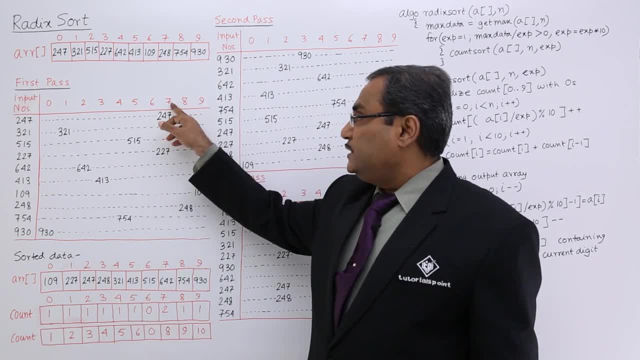 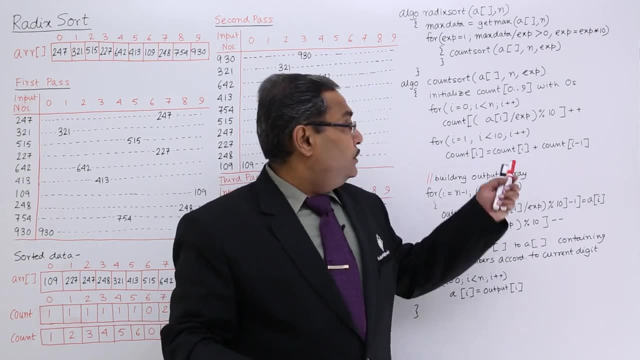 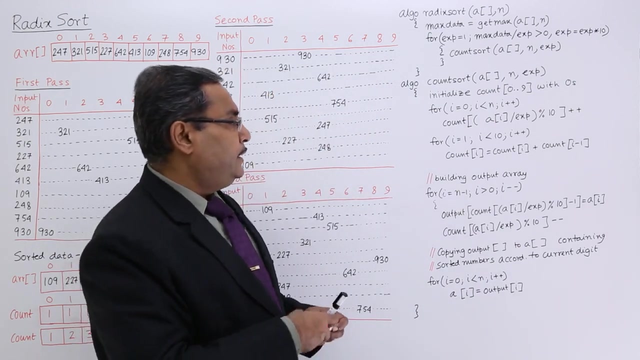 particular for loop: See for the last digit, 7. I am having two numbers, So that is why 7 is having the count value 2.. Done 2. 2. particular code is preparing this count array in this way. next, i am concentrating this one. 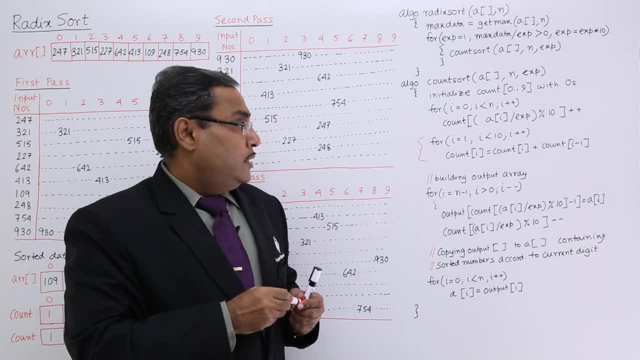 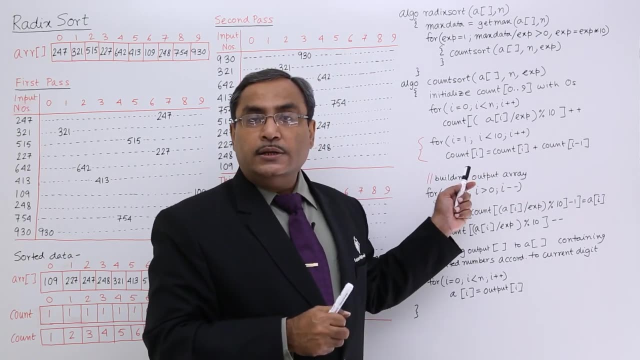 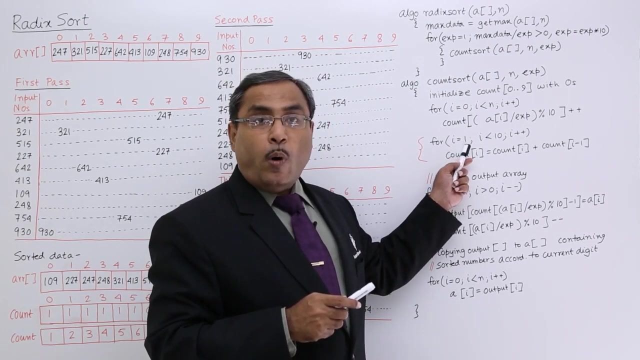 now i am concentrating this one. now they are doing that. count i plus, count i minus. one will be added and that will be assigned to count i. so they are going for cumulative frequency. they are going for cumulative frequency where i is ranging from one to nine. i is ranging 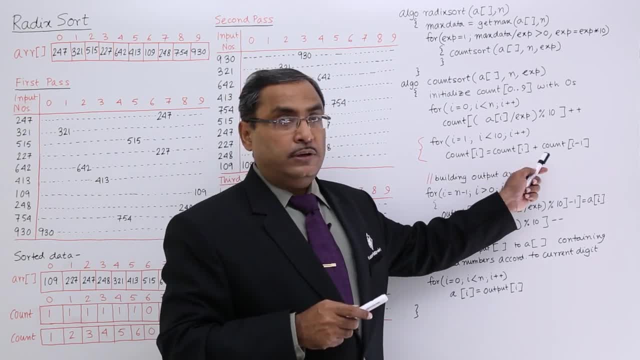 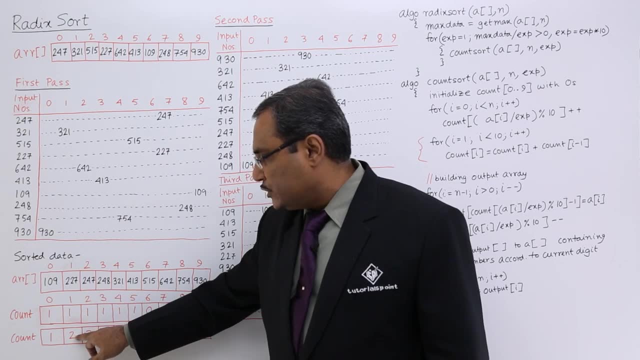 from one to nine, so now they are going for this particular thing. now what will happen? i am just: i have written this one here. see, this one and this one will get added and that will be the new content of location number one. this two and this one will go on adding. 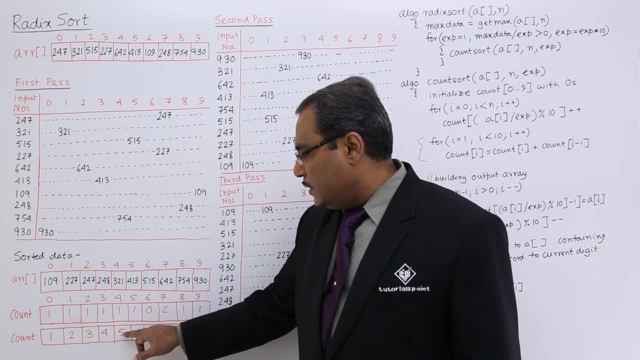 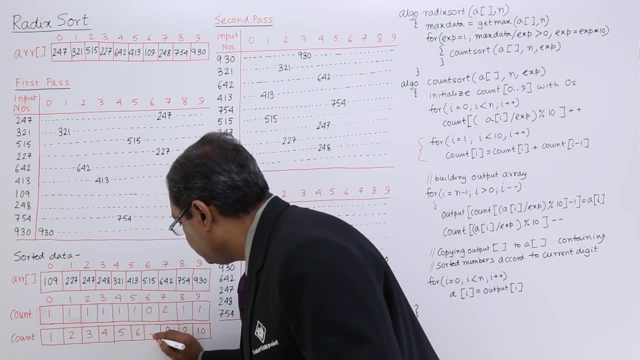 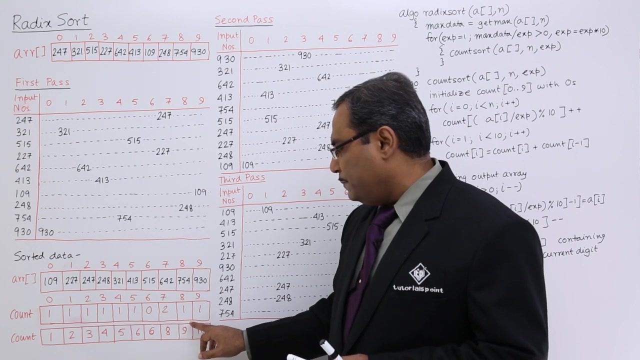 i am getting three, this three plus one, four, this four plus one, five, this five plus one, six, this six plus zero. i should be having a six. okay, now, this six plus two. i should be having eight, eight plus one, nine, nine plus one, ten. obviously, the last one will be ten. 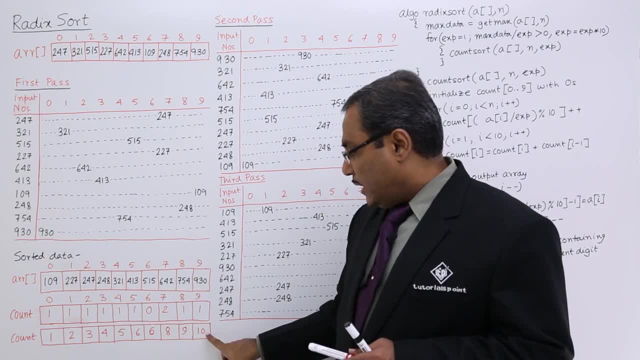 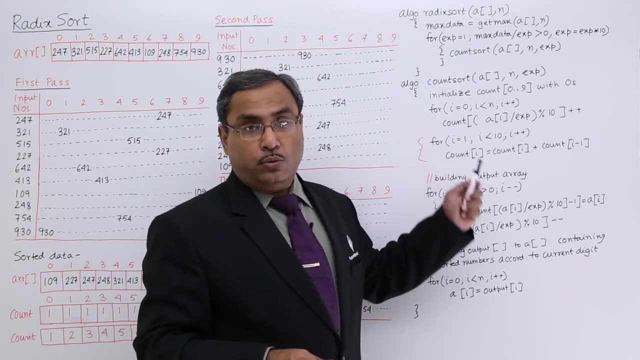 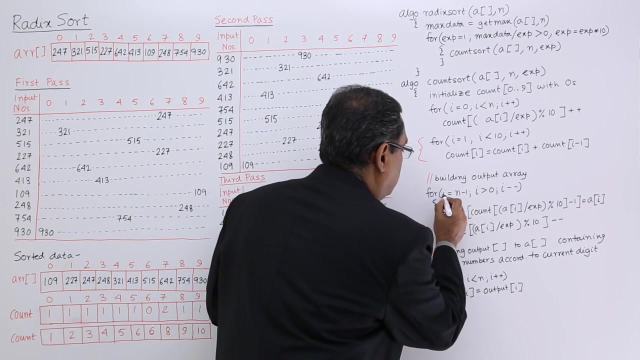 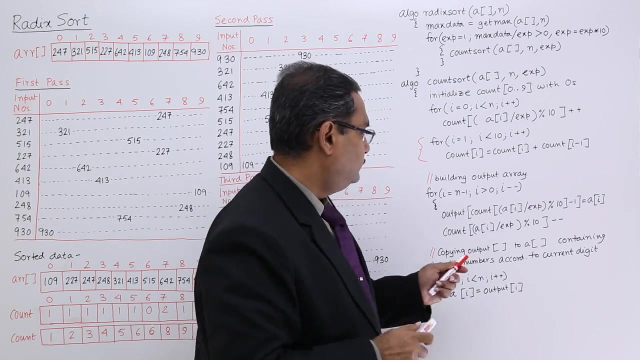 because i was having ten numbers. so that is why the counting will be ten at the last. okay, so this count update has been done in this particular code. so remaining with this particular four, let me discuss that one now. now for i is equal to n minus one. i greater than zero. i minus minus. remember i am reading. 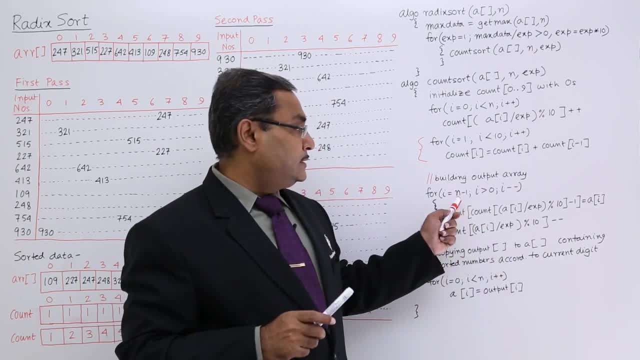 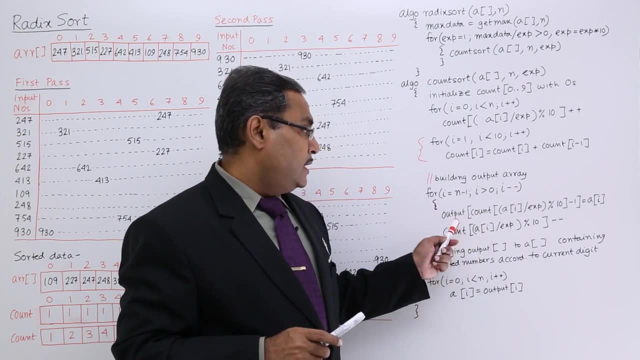 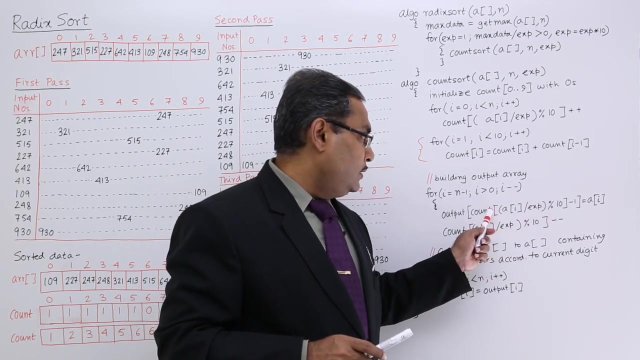 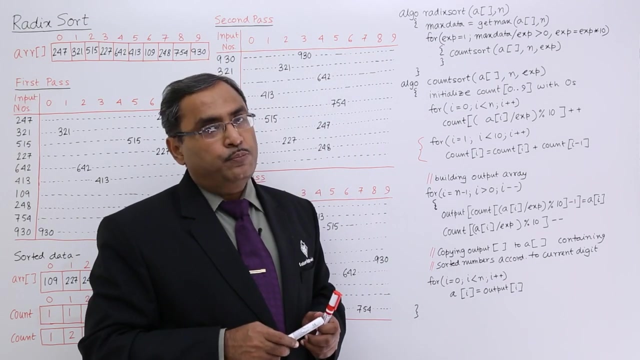 this numbers from the last to first. i am reading this number from last to first. so i is less, i is n minus one, i greater than zero and i minus minus output. count a i by exp percentage. ten minus one output is the array. at that very location i am putting a i. at that very location i am. 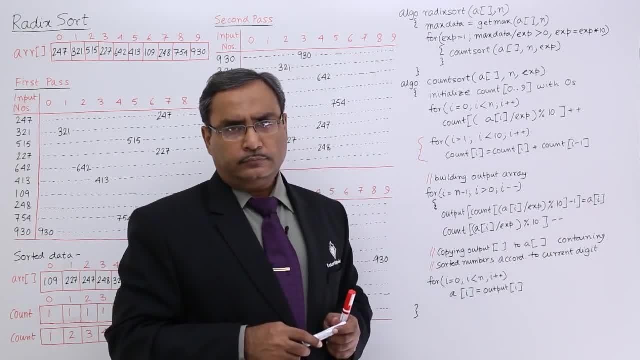 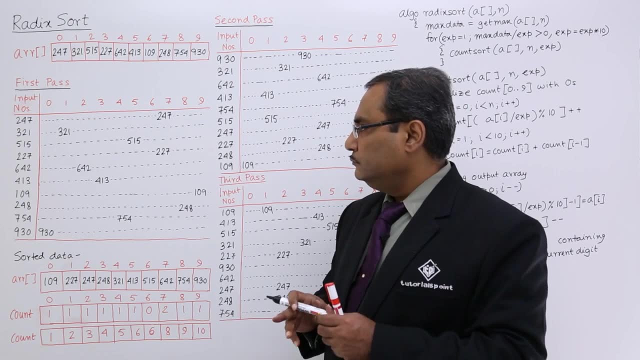 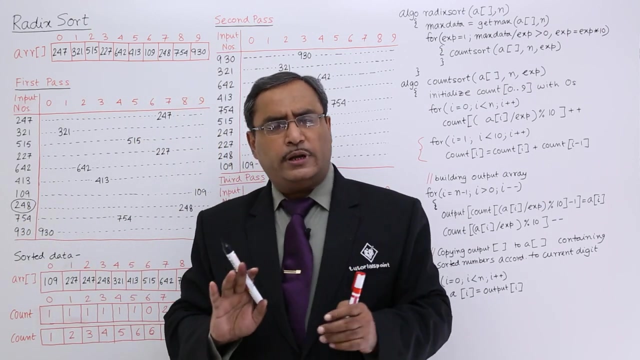 putting a i. so i am putting a i at this particular location. let me go for one example. okay, now take one example. say: say, i am taking this two forty eight. i am taking this two forty eight arbitrarily. i have taken, i am not. i do not know what is going to happen, so two: 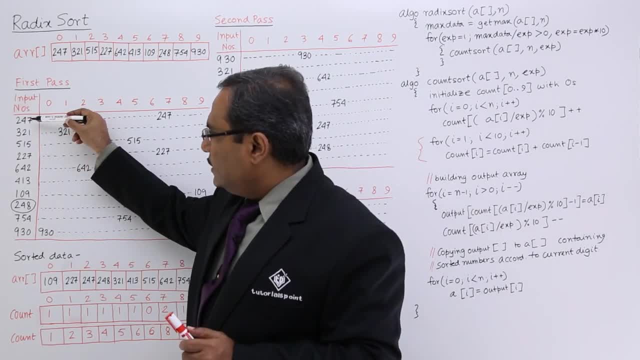 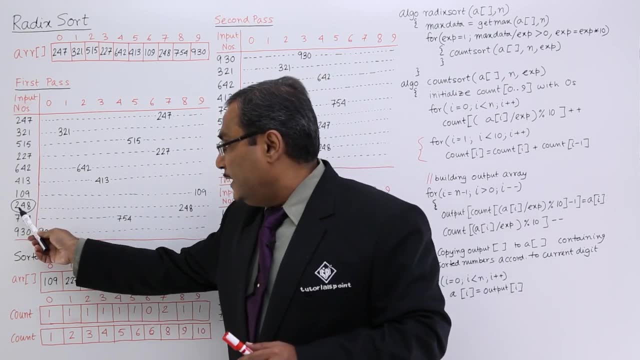 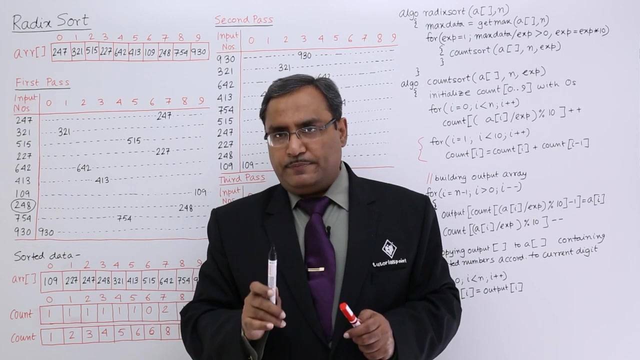 forty eight i have taken. okay, now tell me the subscript in that case. so it is nothing. but it is nine, so it is eight, it is seven. so when the value of i will be seven, then i shall get this a i as two forty eight. okay, let us suppose exp is equal to one for the first time. so two forty eight. 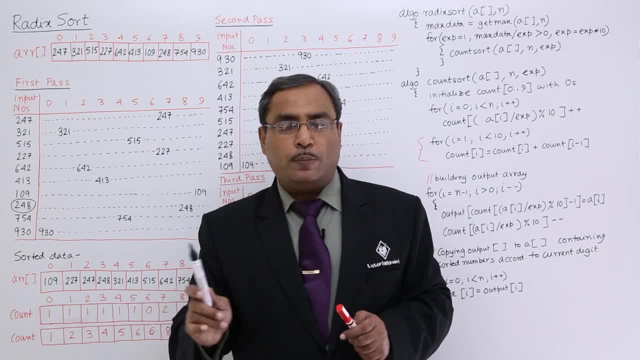 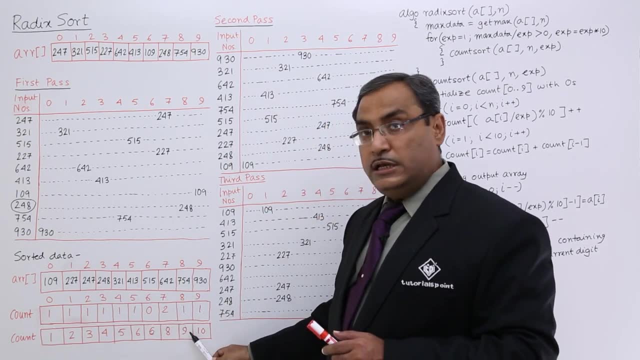 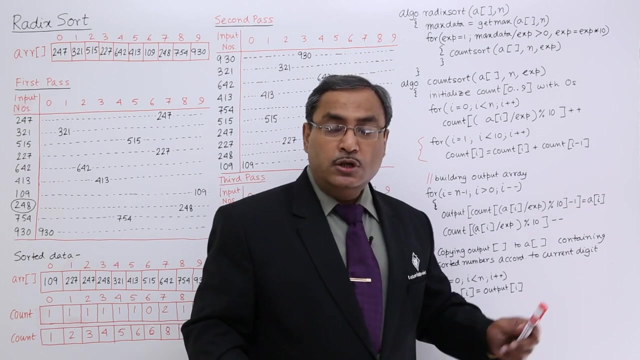 by exp. by one means two forty eight mod of ten. i am getting eight. good, so please come to the count array at the eighth location. what are you getting? you are getting nine. please make nine minus one. please make nine minus one, please. so what is that eight? so 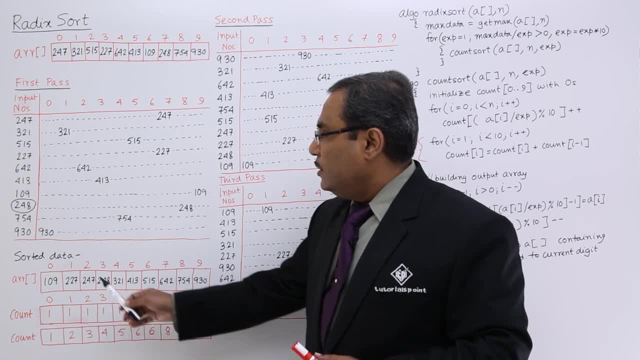 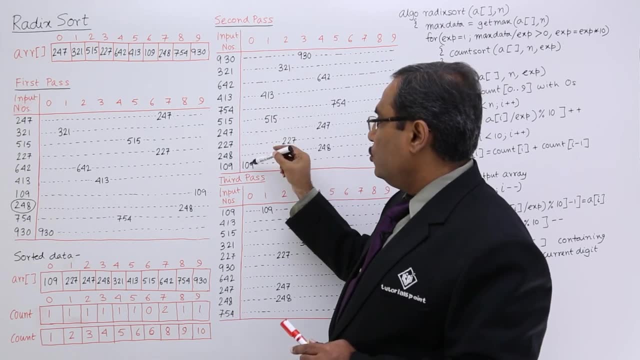 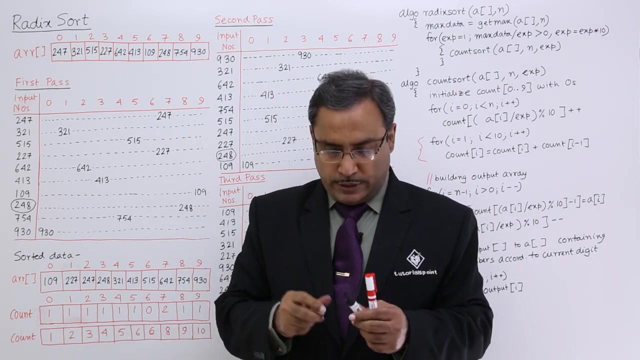 the output array eight. output array eight location will be having this particular two forty eight. let me go for that zero. one, two, three, four, five, six, seven, eight. two forty eight is there at the output array eight. let me go for another choice. let me check whether it is working properly or not. 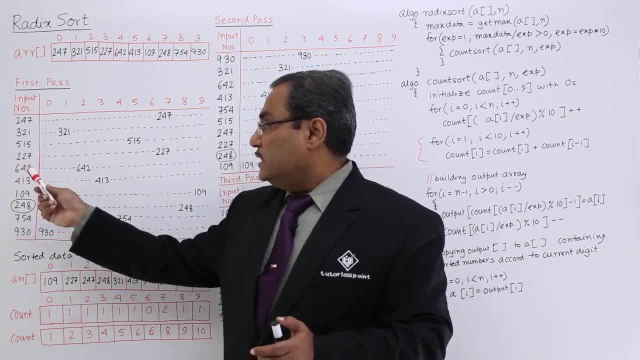 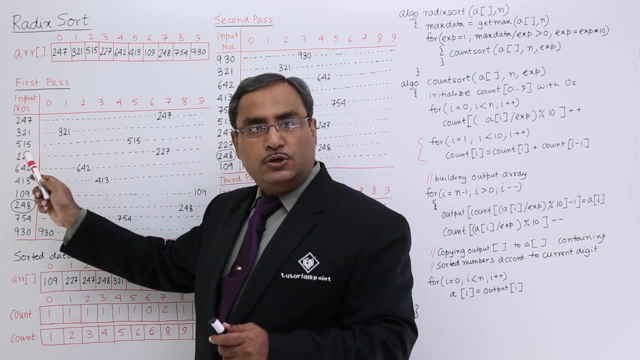 okay now. So what is the value then? i of i is 0,, 1,, 2,, 3.. When the value of i will be 3,, then I am having this: 2, 2, 7.. When the value of i will be 3,, then it is 2,, 2, 7,. good Now. 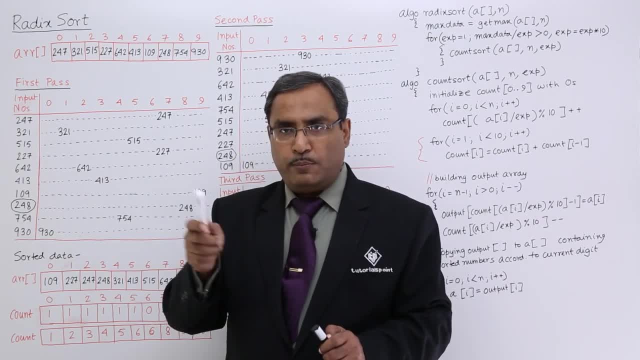 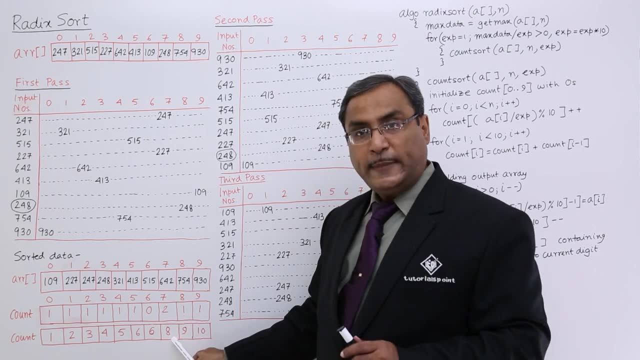 see. please tell 2,, 2, 7 by 1, 2, 2, 7, mod of 10, 7.. Please count. come to this array, count seventh location. What are you getting? 8.. Please make 8 minus 1, 7.. So now at the 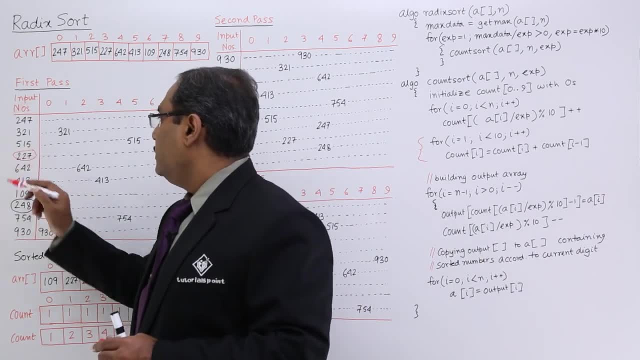 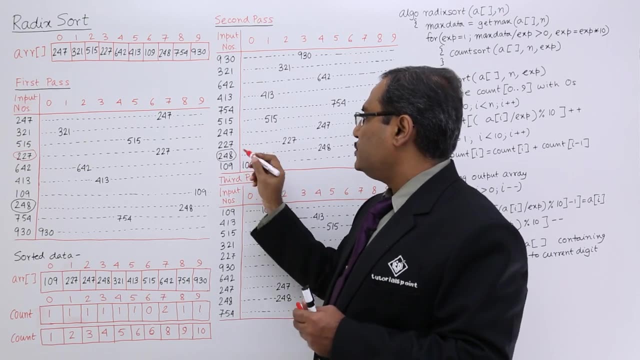 seventh location. I was dealing with this. so at the seventh location you must be having this: 0,, 1,, 2,, 3,, 4,, 5, 6,. at the seventh location you are having this And also you are decreasing. 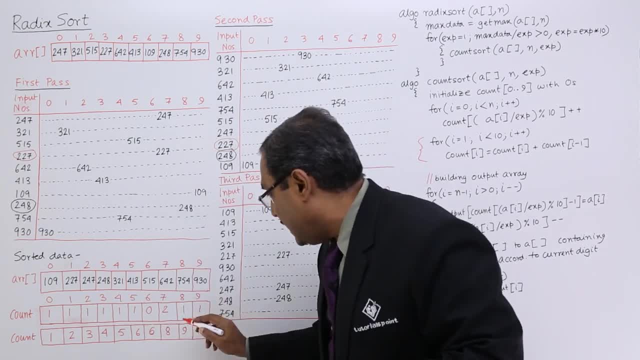 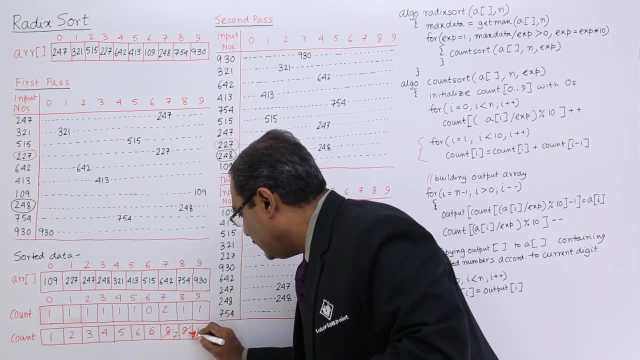 the value of this. also, you are decreasing this value of this. So at the seventh location it will become 7 and initially at the previous case study it will become 7, so it will get decremented by 1.. 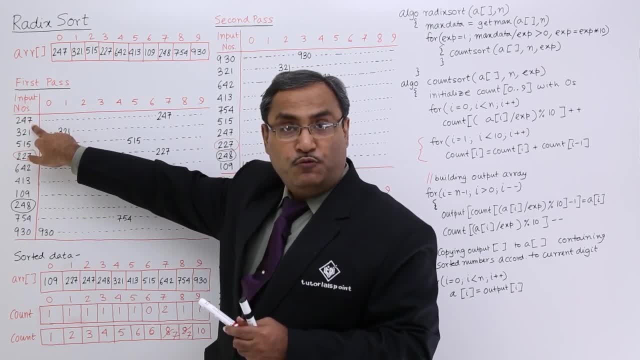 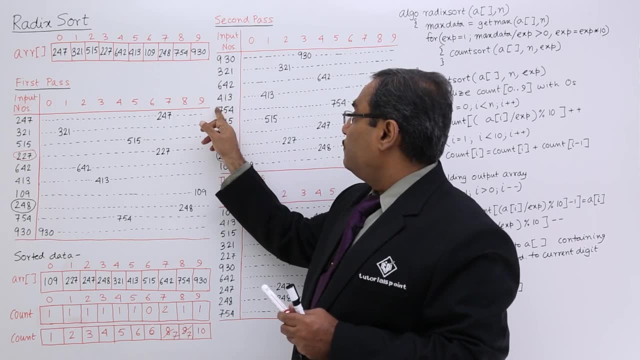 So next time when another last digit 7 number is 247 will come and that will go to the 7 minus 1 6th place: 0, 1, 2, 3, 4, 5, 6 place. yes, it will be going to the 6 place and if, in this way, if you trace, 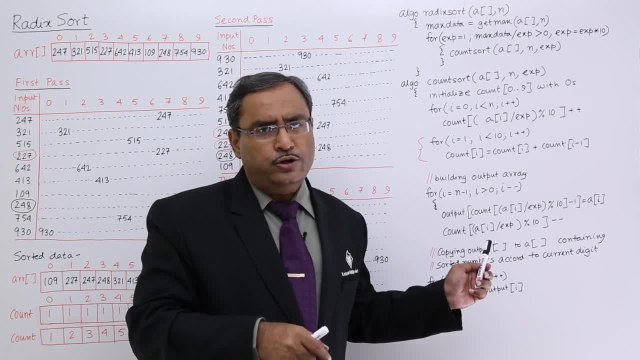 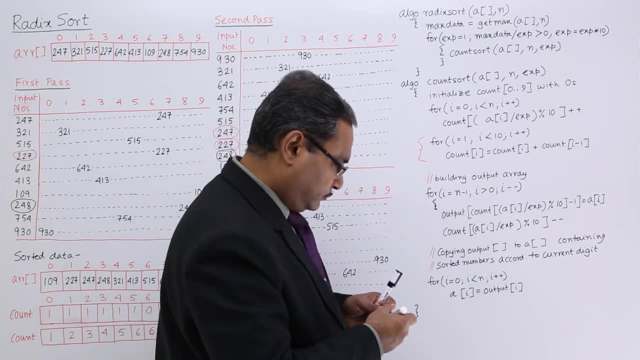 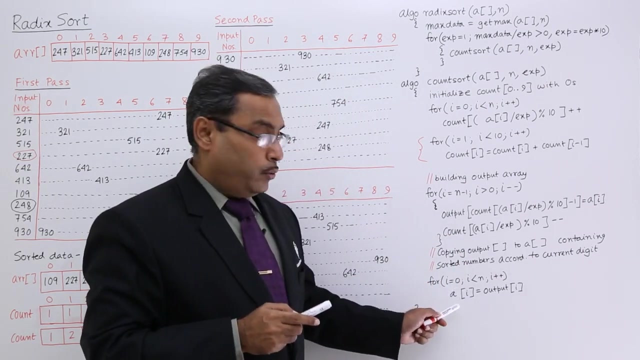 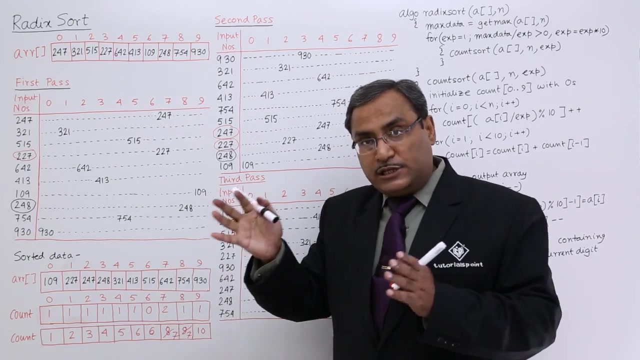 this particular algorithm, each and every line will match according to your logic. so now, in this way they are going this: now this particular algorithm will get terminated. ok, now we are having this particular line where the output will be dumped on to the a: what is output. that means this is the order in which i am reading. i am keeping this one. 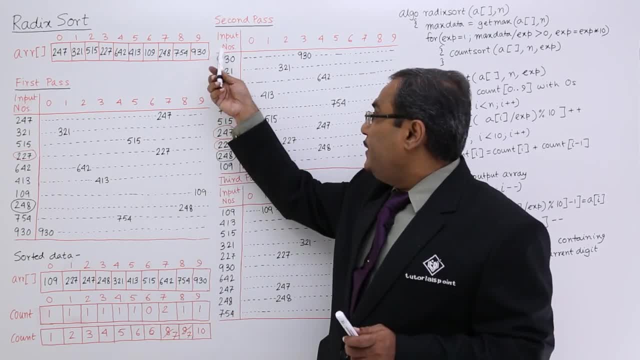 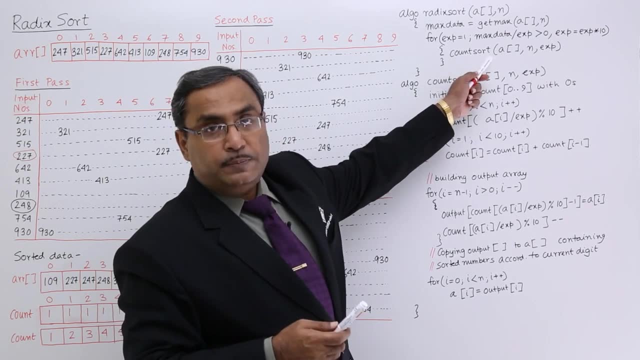 in some temporary array output and the output content will be dumped on to the array a, so that now it will work with this particular array. so now again. next time it will work with that particular array. in this way this radix shot is working. see, this is my algorithm.